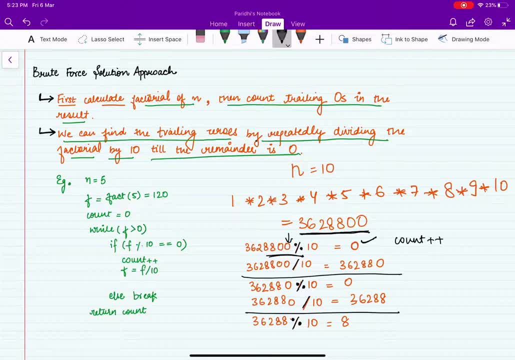 simply increment our count. Next we will divide the number by 10 to check the next number, the next digit. that means this number. So after dividing it we will get nothing but 362880.. So that means this digit has been removed. the last digit Now. we have got this Now in the next iteration. 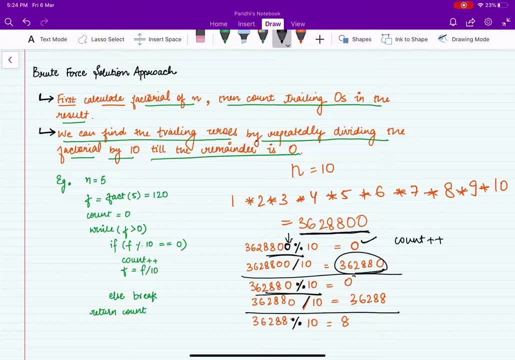 we will simply do the mod of it to get the last digit. We got it as 0.. So again, we will increment the count. Next, we will divide it by 10.. So here we have divided it by 10.. Next we will divide it by 10.. So here we have divided it by 10. Now in the next iteration we will simply do the mod of it to get the last digit. We got it as 0. So again we will. 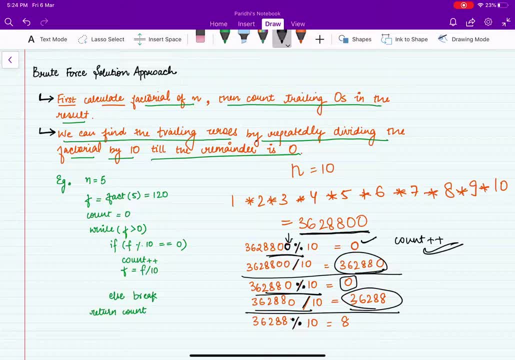 increment the count. Next we will divide it by 10. So here we have divided it by 10. So it by 10 again. find the mod of it and we get a non-zero number. that means here we have to stop. 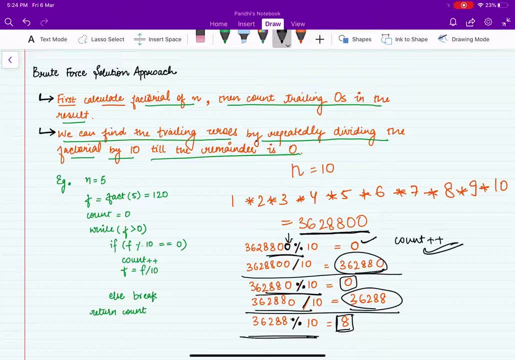 because we have find, we have found out all the trailing zeros and since we have got a non-zero numbers, that means we do not care what is there at the left of it, right, so we will simply stop and return the count and this is what written in this snippet: that we have got the factorial as. 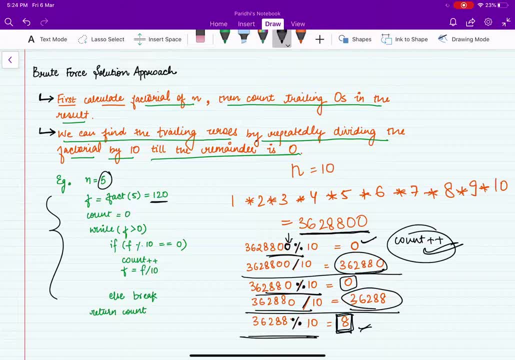 120 of 5 when n is 5. so we will run our loop till this factorial is greater than 0. so if f mod 10 is equal to is equal to 0, we will simply count it up and we will divide f by 10. 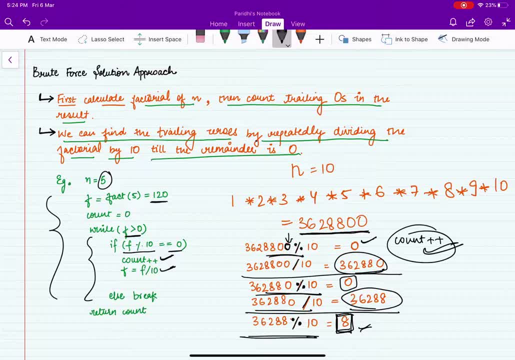 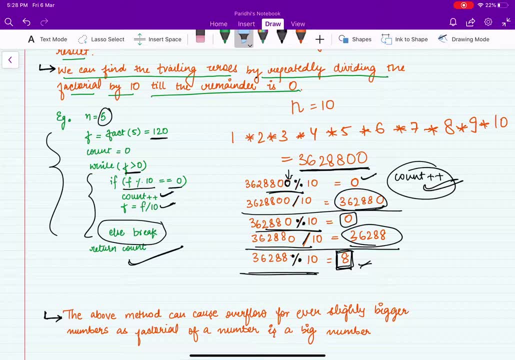 and else, if it's not 0, then we will simply break because we do not care what is there on the left, and we will simply return the count. but the problem with this approach is that the above method can cause overflow for even slightly bigger numbers, as the factorial 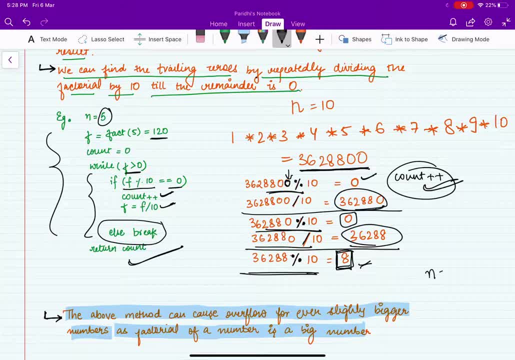 of a number is a big number. so even if the number is as small as, let's say, 22, then it's going to cause overflow because the factorial of a even a small number is so big that it can. it is certain to cause overflow, right? therefore this method is not the appropriate one. 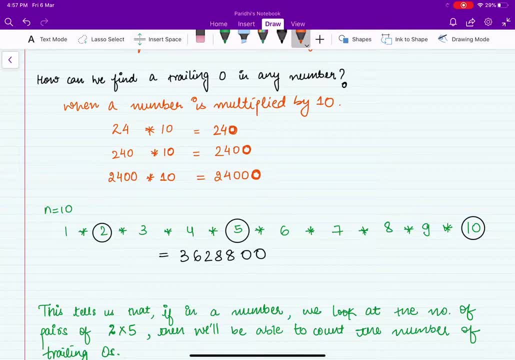 so what should we do now? let's see what is a better approach. so how can we find a trailing zero in any number? how can we do that? so when a number is multiplied by 10, we get a trailing zero, right? so let's see 24. if it's multiplied by 10, we get 240. 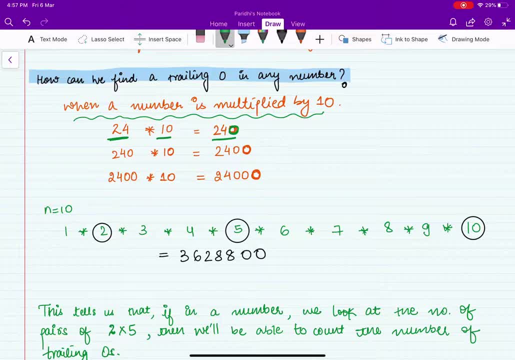 so. so here we have got a trailing zero. just because we have multiplied it by 10, then we have, let's say, 240, and if we multiply it by 10 we get to 2400. we have got another zero which is contributed by this 10 right. so in 2400, if we do into 10, we will get 24000. so another zero which. 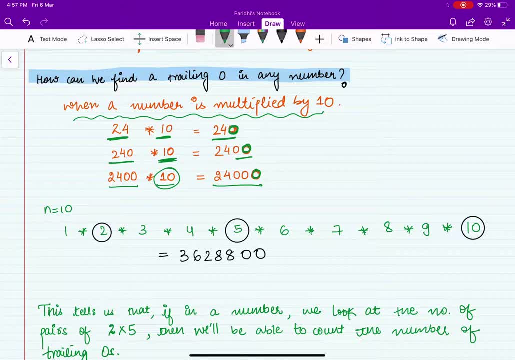 is contributed by 10. so here there is an observation to make that a number, if multiplied by 10, by 10, it will give us a trailing zero. so, for example, if n is equal to 10, then we'll get this as the. this is the factorial of 10. so 1 into 2, into 3, into 4, into 5, into 6, into 7, into 8, into 9, into 10. 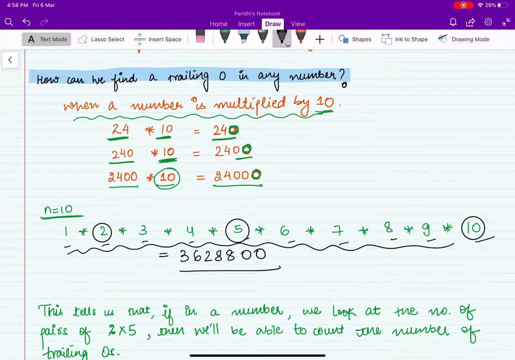 the factorial is this: and we can see that there are two zeros, the two trailing zeros. that means there must be number two tens. right, there must be number of 10. tens is equal to 2 that are contributing to two zeros. so how are we getting that? so 110 is here and 110 is formed by the. 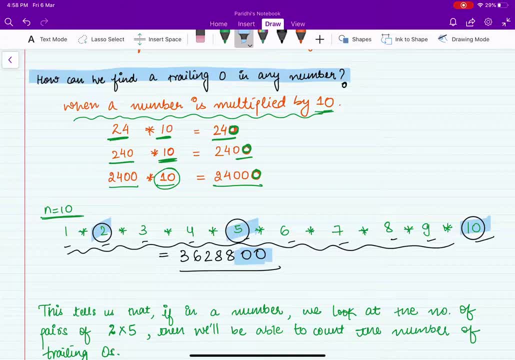 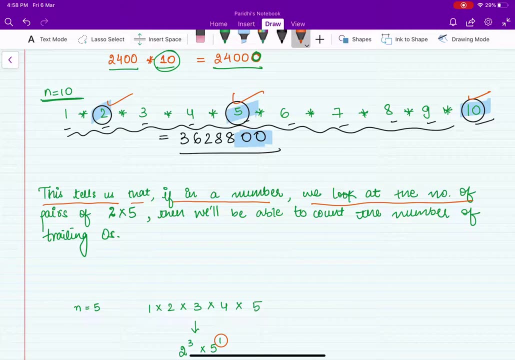 combination of 2 and 5. so if you multiply 2 and 5 we'll get 110 right. so this is 110 and we will get 110 from here, so that accounts to two zeros. so this tells us that if in a number we look at the number of pairs of 2 into 5, then we'll be able to count the number of trailing. 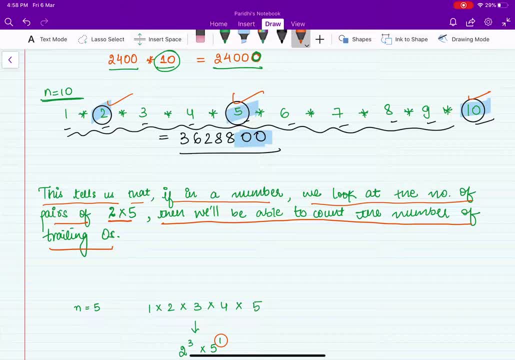 zeros. so if, if in a number we look at that, how many number of twos are there and how many number of fives are there, then we take the smaller number, we take the power, the smaller power of a number. let's say 2 is x and 5 is y. so let's say y is smaller than x, then we will take. 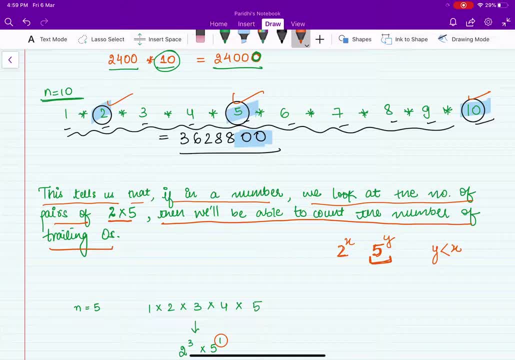 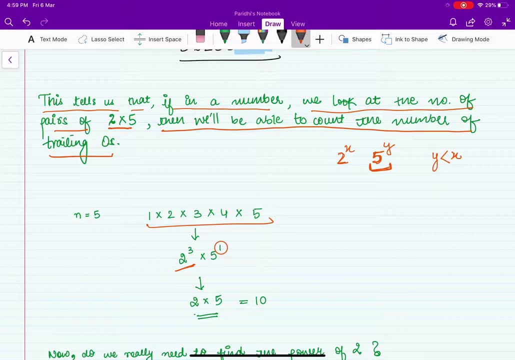 this the number of fives, and that is going to be the answer why? because let's see with the help of this example. so in this case the power of 2 is 3. that means there are the three, twos, there are number of twos as 3, so this is 1, and 2 into 2 gives us 4. so 1, 2, 3, so there are two, threes and 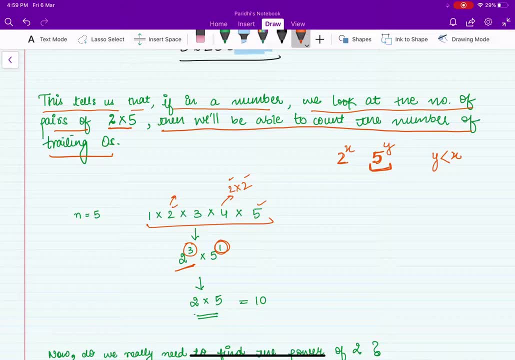 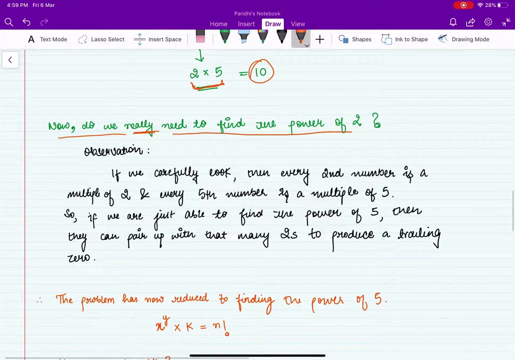 5 is just 1, right, so 5 will pair up with a single 2 to form a 10. therefore, we will look at a lesser 2 and 5 right now. do we really need to find the power of 2? do we really need to find a power of 2? 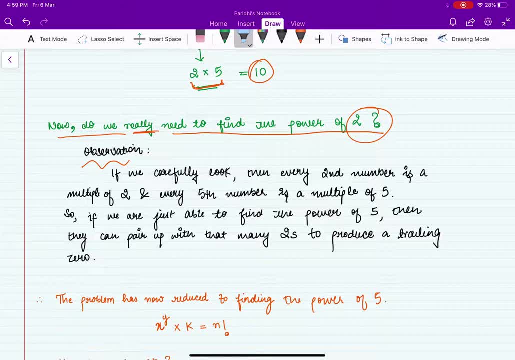 well. here the observation is to be made that if we carefully look, then every second number is a multiple of 2 and every fifth number is a multiple of 5. so if we are just able to find the power of 5, then they can pair up with that many number of twos. so if we look carefully then we 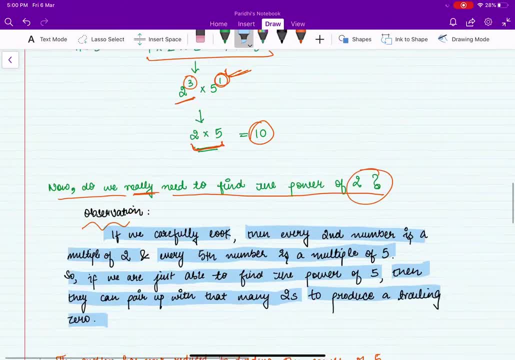 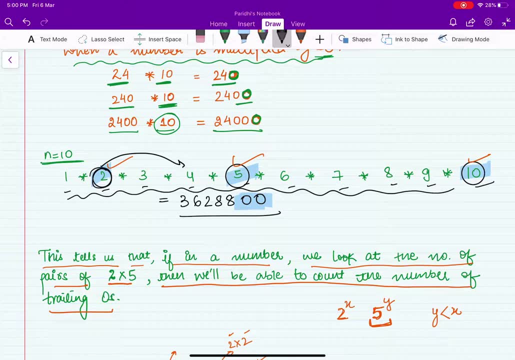 can see that there are combinations of five, number of twos which are going to be 저는 above with the help of example. so in this case, every alternative number. so this is a multiple of two, then this is a multiple of two. six is a multiple of two. eight is a multiple of two. 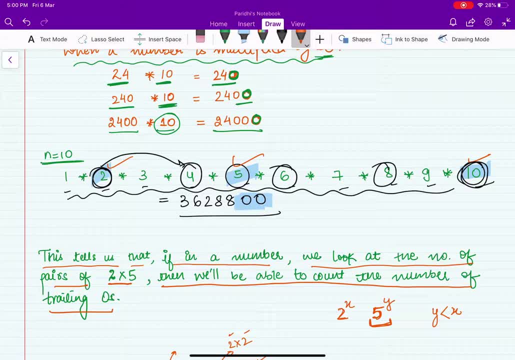 then 10 is a multiple of two. so at every second number we are able to find the multiple of two, which will give us the number of two. right, that will give us the number of twos. and every fifth number, every fifth number is going to be the. 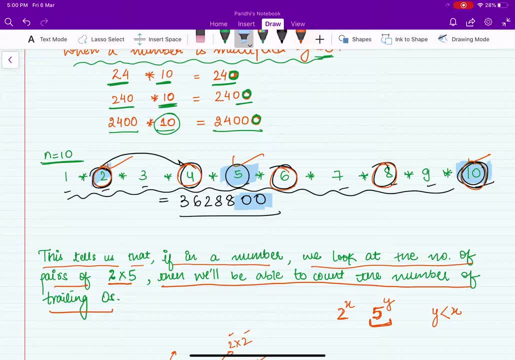 multiple of 5. that will contribute to a power of 5. right, that will contribute to the power of 5.. So, as we can see that the number of multiples of 2 are greater than number of multiples of 5, that means we are going to get more number of 2s as compared to 5.. So the number of 2s are going. 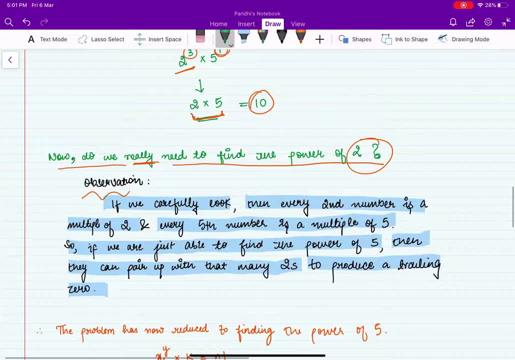 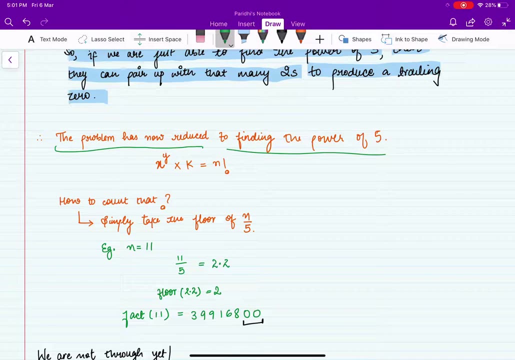 to be greater as compared to the number of 5.. So we need not calculate the power of 2. instead, we can simply calculate the number of 5s or the power of 5.. So the problem has now reduced to finding the power of 5.. So this is a generalized equation, like if we want to find a power of any. 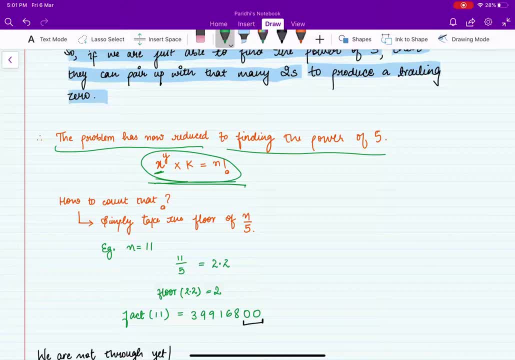 number, then we can apply this formula Here: our x is equal to 5.. So here we are actually trying to find the power of 5 and let this be any number, the remaining number, which, when multiplied with power of 5, gives us factorial n. 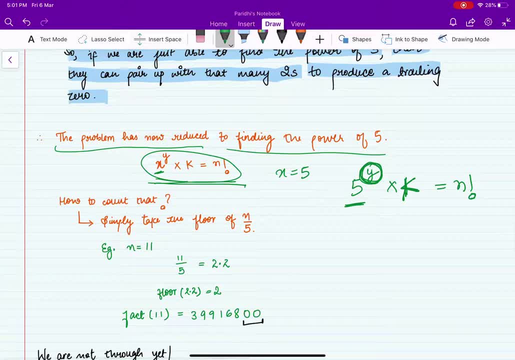 So how can we find the power of 5 or how can we calculate the number of 5?? So for that purpose we can simply take the floor of n by 5.. For example, let's say n is equal to 11.. Now n by 5. 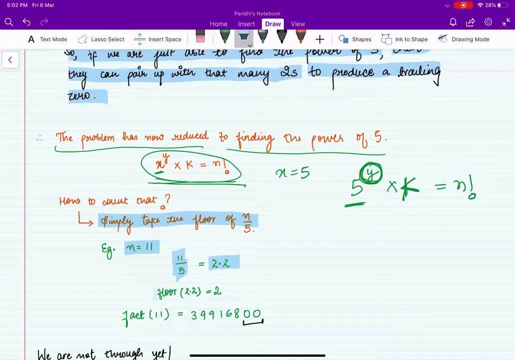 gives us 2.2. The floor of 2.2 is nothing but 2.. That means the factorial of n is going to have two zeros. If we see here, then the factorial of 11 is nothing But 3,, 9,, 9,, 1,, 6,, 8, double 0. So there are two zeros, The two trailing zeros, Because in 11, how? 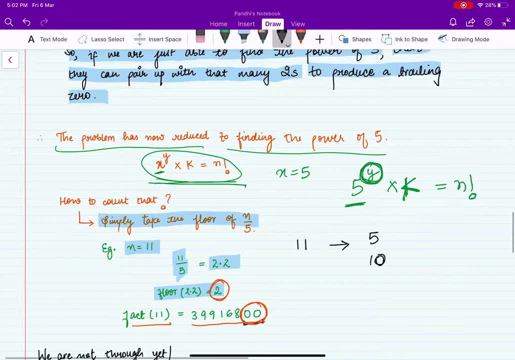 many multiples of 5 are there. It's 5 and 10.. So this has contributed to 1, 5 and this has contributed to 1, 5.. Therefore, the total number of 5s are 2 and therefore the trailing zeros are 2.. 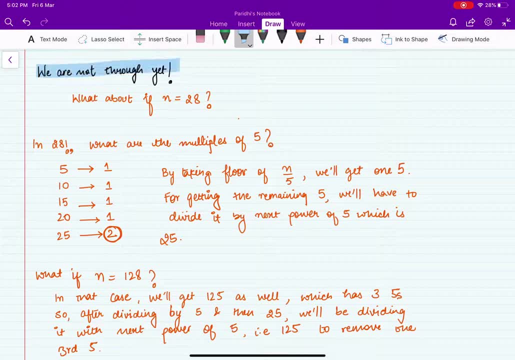 But we are not through yet. Why? Because what about if n is equal to 20? What will happen in that case? So if n is equal to 28.. So, in 28 factorial, what are the multiples of 5?? So the multiples of 5 are 5 itself, then 10,, 15,, 20 and 25.. 5 will contribute to 1, 0. 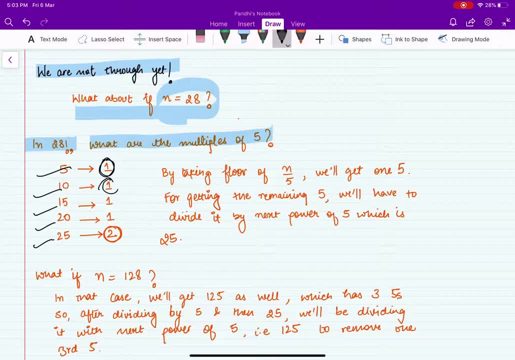 10 will- sorry, 5 will contribute to 1, 5.. Then 10 will contribute to another 5.. 15, another 5.. 20 will also contribute to 1, 5.. But here 25 is going to contribute to 2, 5.. 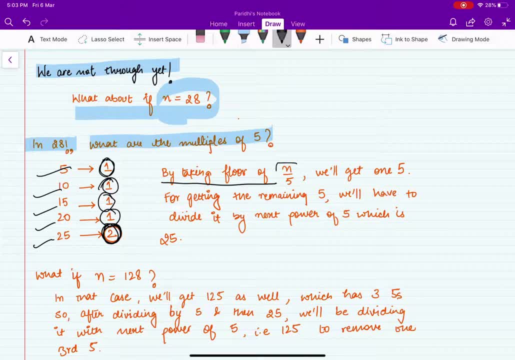 So by taking floor of n by 5 with the formula n by 5 and taking floor of it, we'll get 1, 5.. So if we do n by 5, that means 28 by 5. this is going to give us 5 only. So that means here we. 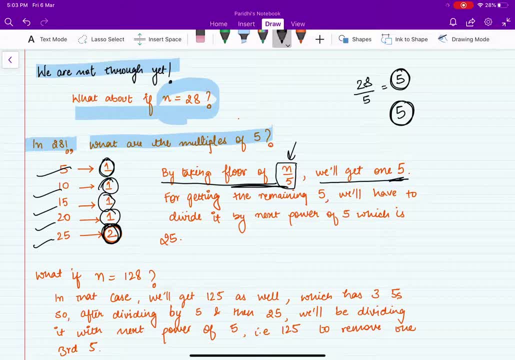 are going to get just 5 zeros, But here we can see that there are 6 zeros in total. So for getting the left out 5- that means the 5 which is to be counted- we'll have to divide it by next power of 5, which is 25.. So now we actually have 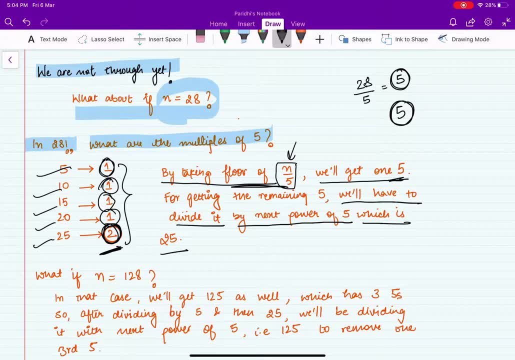 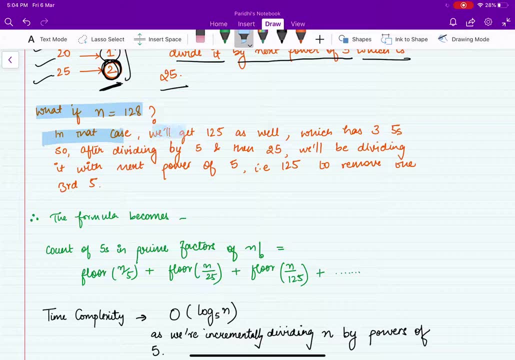 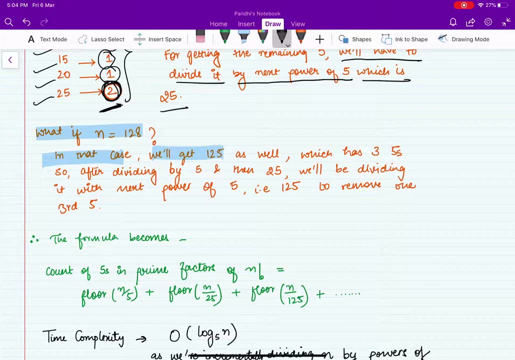 to calculate the power of 25.. But now, what about 128?? So in that case we'll get 125 as well in the multiples of 128 factorial, The multiples of 5 in 128 factorial. So it's going to be 5,, 10,, 15,. 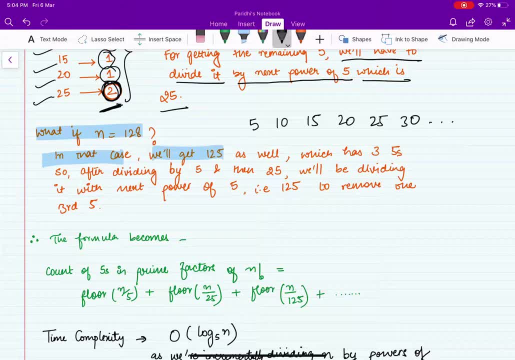 then 20,, 25,, 30 and so on, then 125 as well. So which has so 125 has 3 number of fives. So after dividing by 5 and then by 25, we'll still be left with one more 5.. 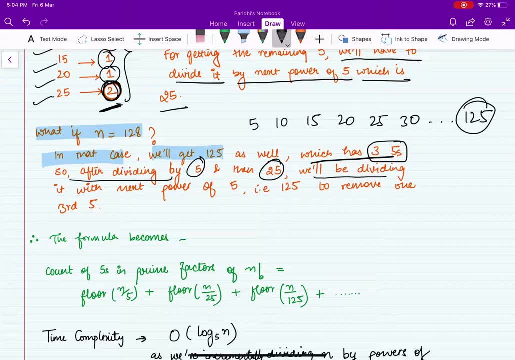 So for that we'll have to divide it with the next power of 5, which is 125, to remove the to actually get the 라unt, the third five. Now the formula has become so: the count of number of fives in factors in prime. 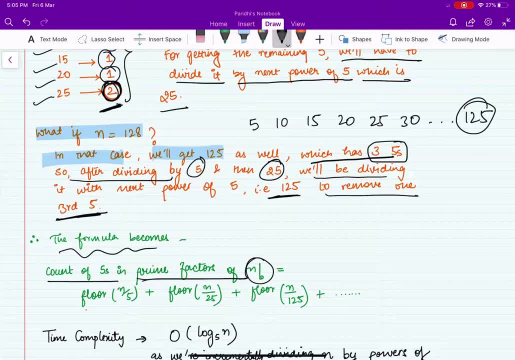 factors of n. factorial, it's equal to floor of n by 5, plus floor of n by 25, plus the floor of n by 125, and so on, till the number is greater than n by power of 5.. So the time complexity of this. 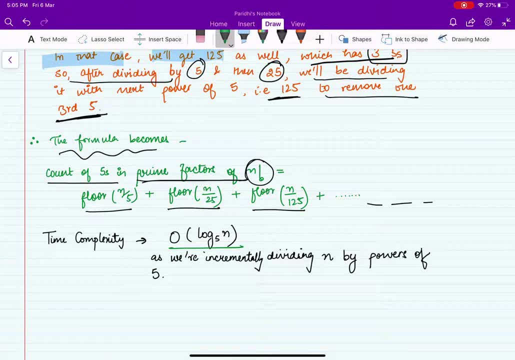 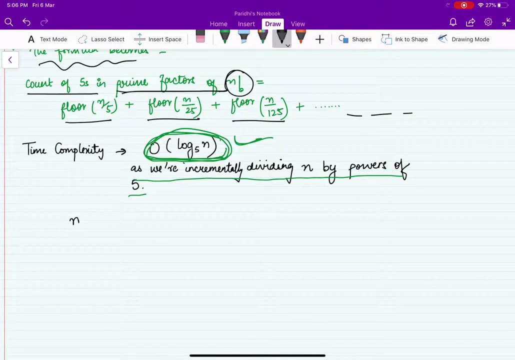 approach is going to be: order of log base 5 n. What was the question? that we have to find a logarithmic time complexity. and we have actually achieved that. So why? because we are incrementingly dividing n by powers of 5.. So first we are dividing n by powers of 5 and second we are 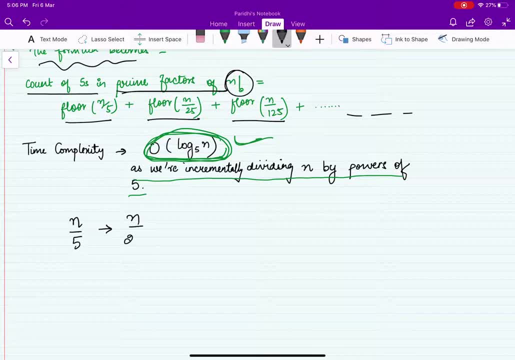 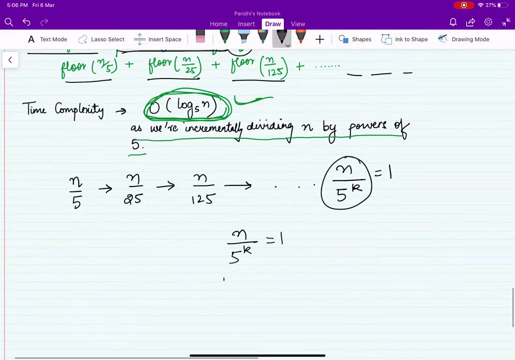 n by 5, then n by 25, then n by 125, so on till n by 5 to the power k, which reduces to 1, and n by 5 to the power k is equal to 1, so n is equal to 5 to the power k after taking log.